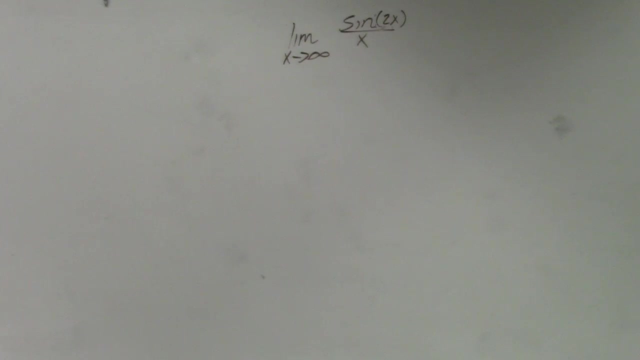 Okay, If you guys look at this, one thing I want you guys to go through, which a lot of you had trouble with on your last quiz, was using the properties of limits. Remember, we can break apart. you know properties And that was one of the things that I'll explain to you. I'll show you. 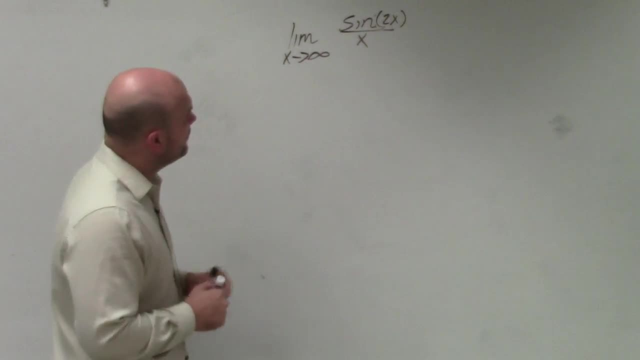 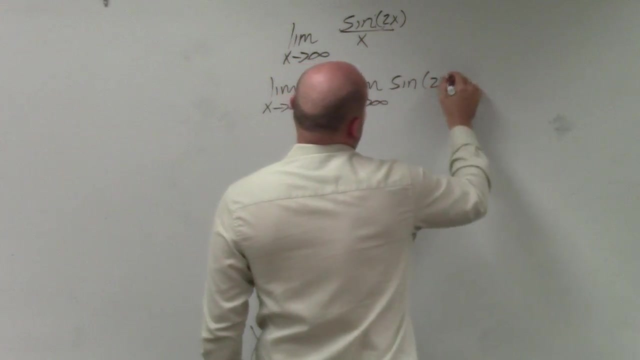 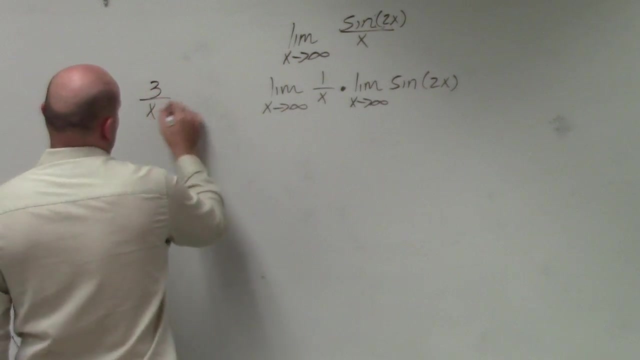 guys in your work. But if you guys kind of look at this, we can break this apart into the limit as x approaches infinity of 1 over x times the limit as x approaches infinity of sine of 2x. Because do you guys agree? Like it's like saying 3 divided by x is equal to 1 over x. 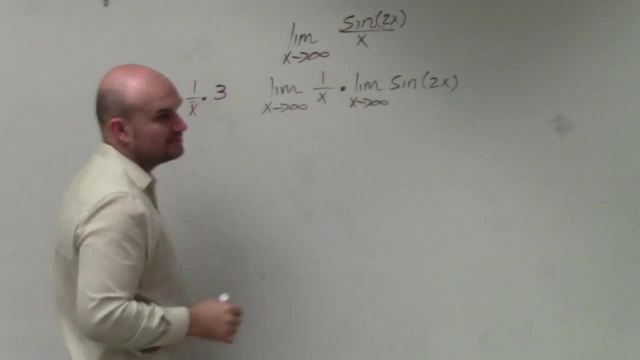 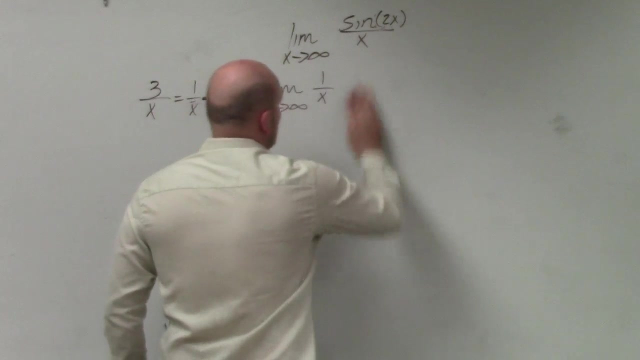 times 3.. Do you guys kind of see how I just did that Now? basically, actually, let me make that very clear. maybe not even go a little bit too fast. You can break that up into the limit of 1 times x times. 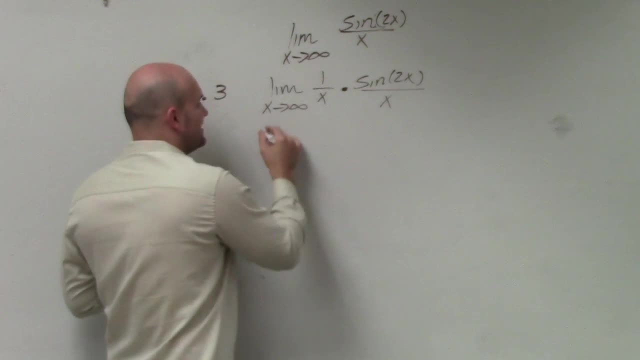 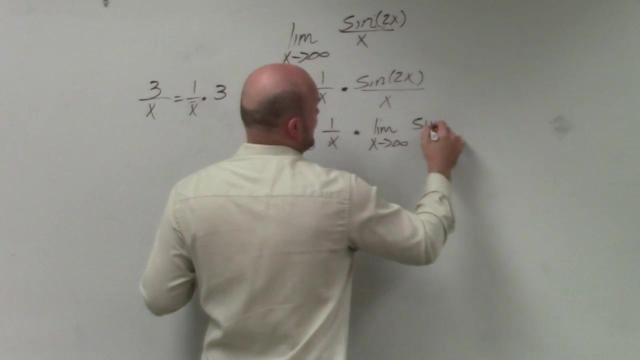 the sine of 2x over x, Then it makes sense to say, oh, when I have the limit of the product, if you guys remember your rules of limits, what that means is I can basically take the limit of them separately and evaluate. 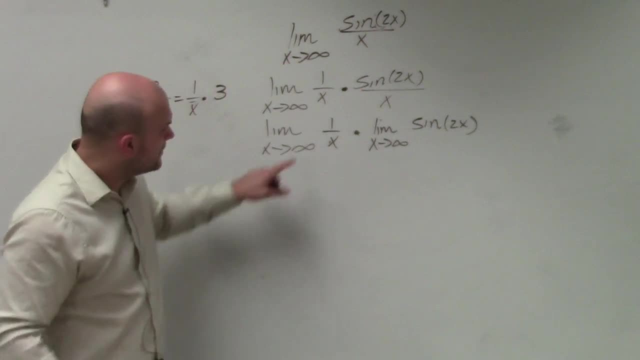 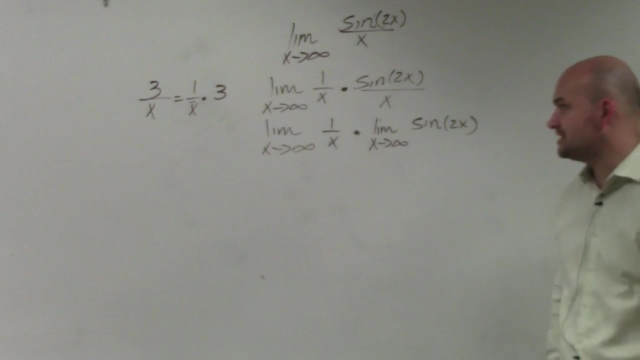 All right now. this one probably would have taken. I actually wanted to go over this before giving you your homework, so I kind of apologize in that regard. First of all, we know what this limit's going to be, which is 0.. 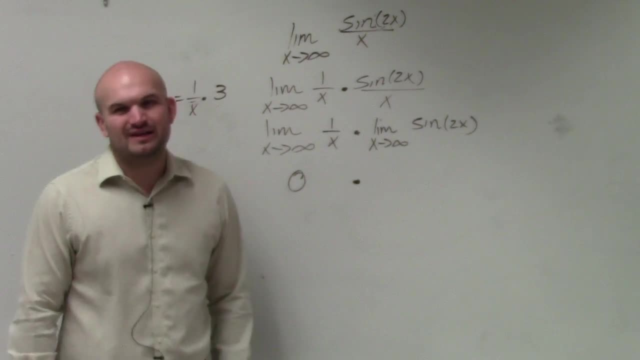 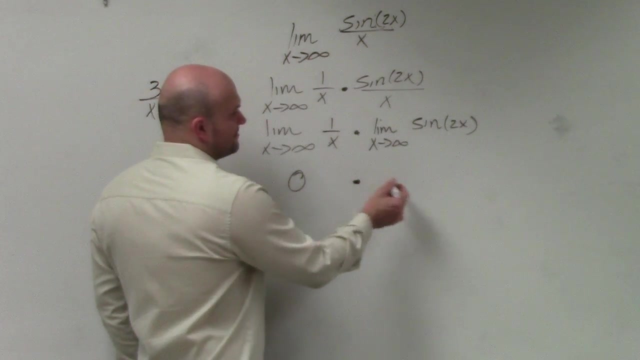 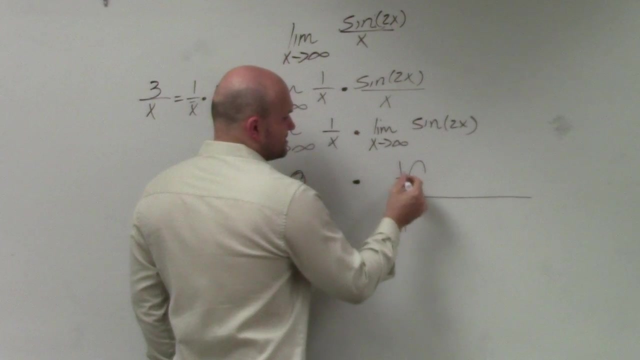 Now we have this limit of sine equals 2x, as x goes to infinity And we didn't get to talk about this and I apologize, But if you guys look at this, this sine of 2x tells you that's going to actually not. 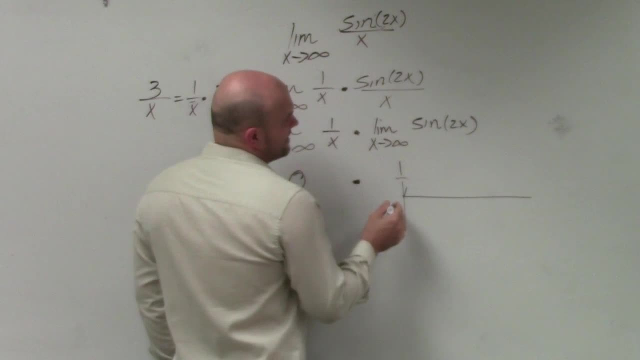 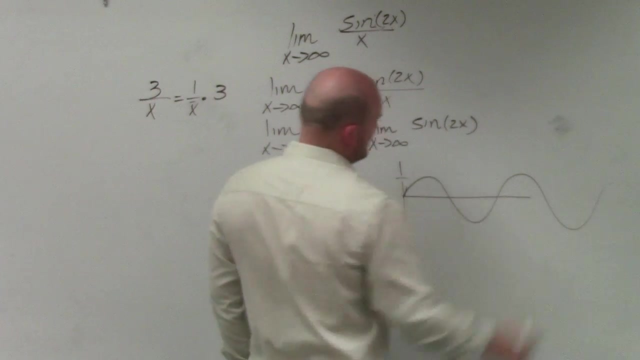 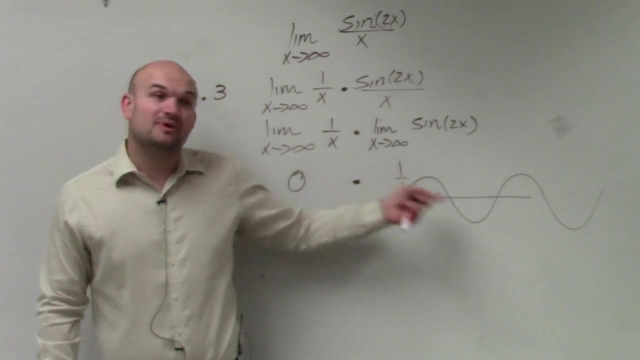 change the amplitude, That changes your sine of 2x. That's going to elongate things, But, if you guys remember, sine looks something like that. So, as it goes to infinity, does it ever approach a number? No, but you've got to think. but what does it approach?